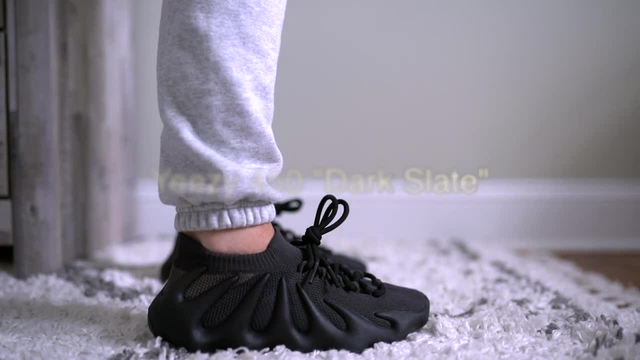 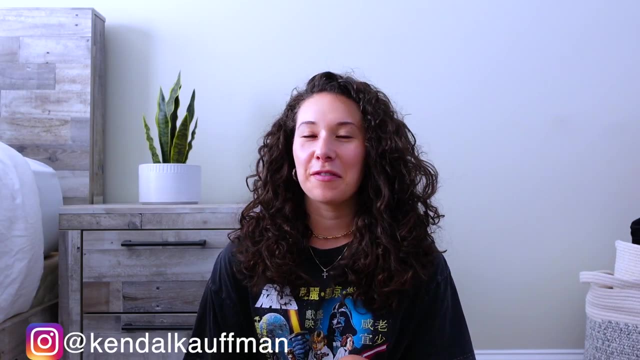 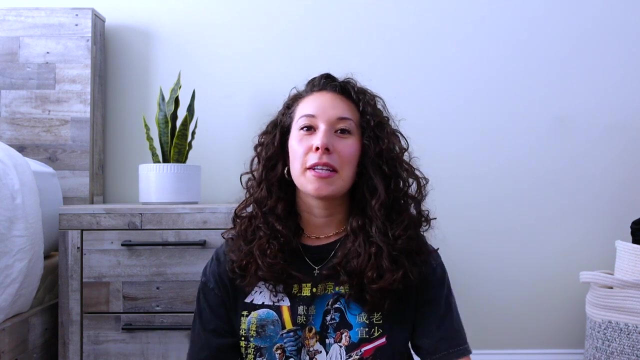 Hey guys, what's up and welcome back. I know it's been a few weeks since I posted my last video, so I have gotten in a few sneakers and I know I actually have been having a little bit of luck with the sneakers lately. I mean just been able to pick up a few, so I'm really excited about it. 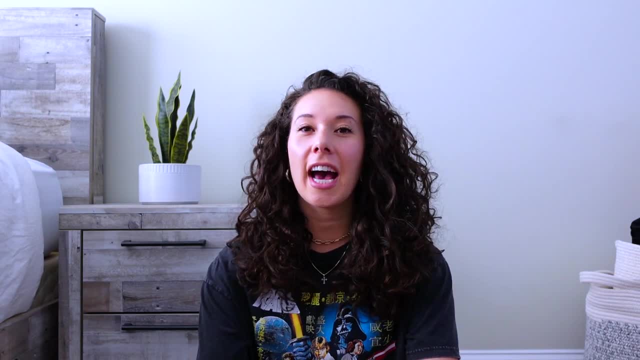 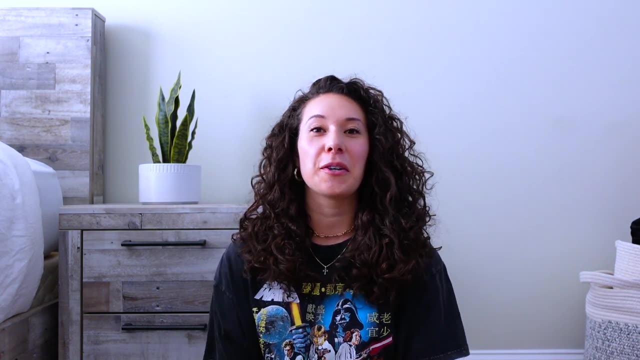 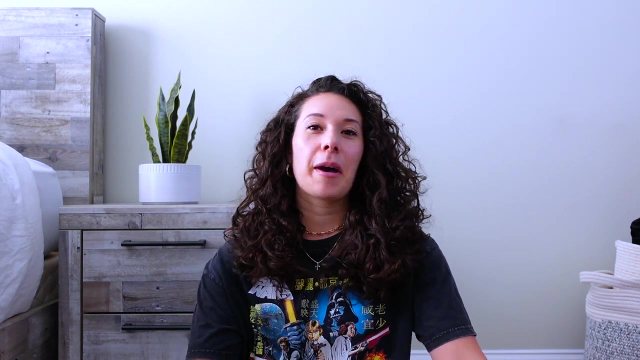 So I do have a few more videos coming. So today I did end up getting the Adidas 450 and I got it in the dark slate colorway, so I'm excited to share them, because it's really different from any of the other Yeezys, I think, anyway. So yeah, I'm gonna be talking about the 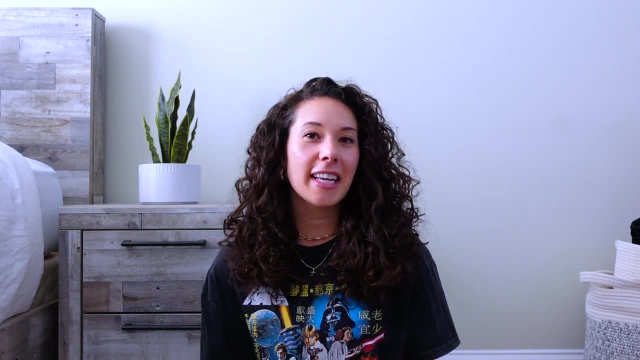 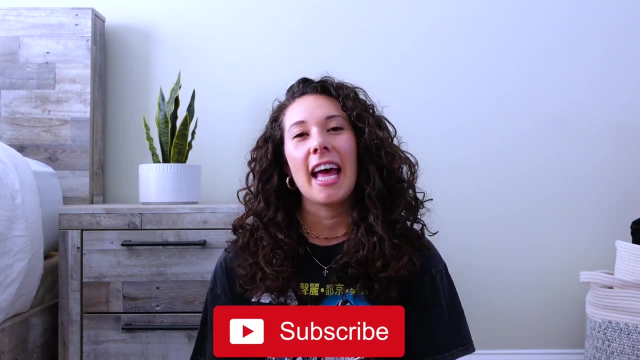 details of the shoe, kind of like the sizing and what I think, and then I will be doing it on foot at the end. So yeah, if you guys aren't subscribed already, make sure you guys hit that subscribe button and let's go ahead and get right into the video. Okay, so, starting off, I do want to talk. 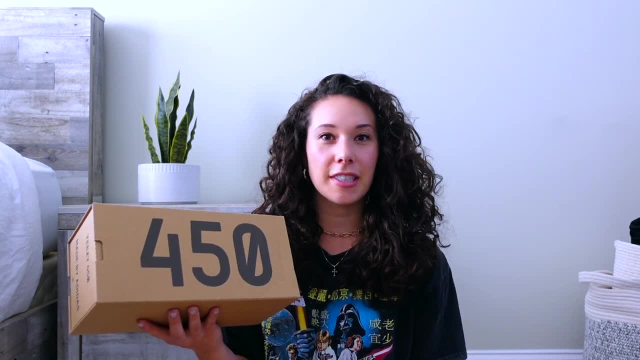 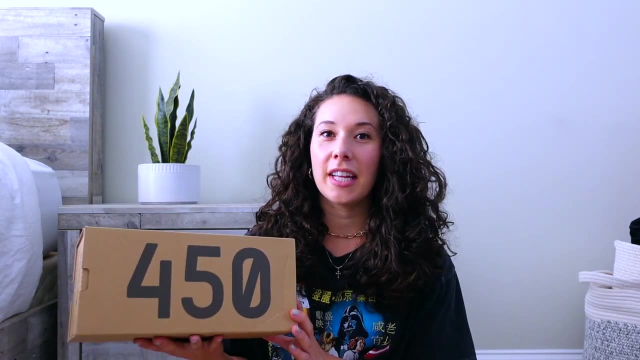 about it. The box is a lot different than the other Yeezy boxes. So if you're used to the 350s or like 700s or even 500s, the box is completely different. It's wider, so I just never really. 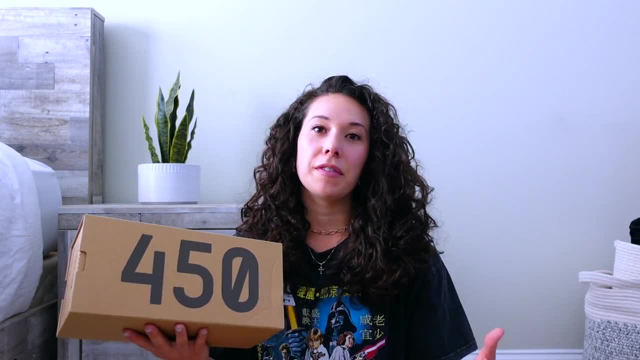 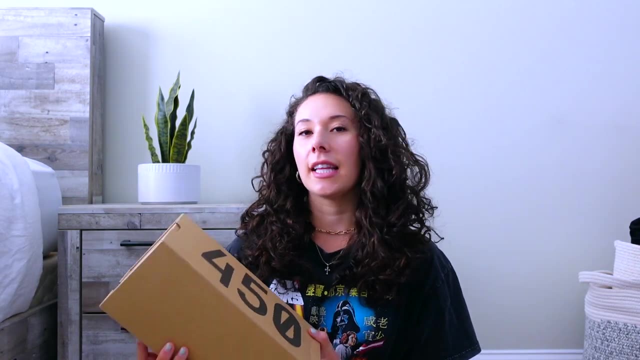 looked at reviews or anything on the 450s so if you would have seen that then you probably would have already known that. So I was able to actually win these on confirmed and lately I feel like I just really like Adidas because they give me some wins on there, Like sneakers app is so hard. 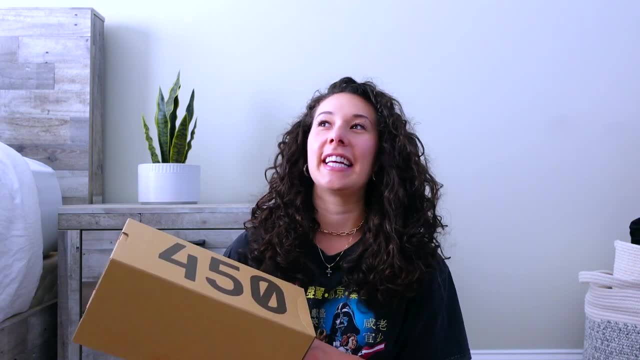 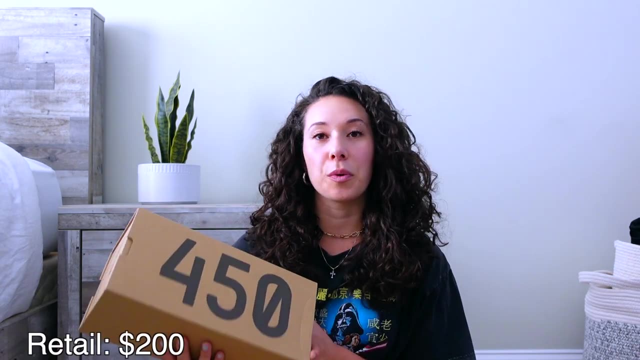 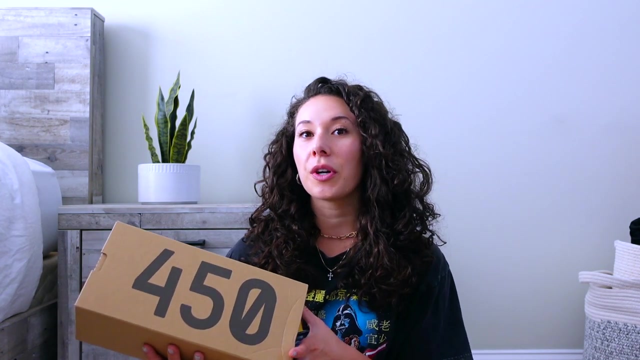 to get any wins, even though I did get my first win in like a year. So yeah, it just feels nice sometimes to get some wins. but I did get these on the confirmed app for $200, and this is actually the second colorway that came out. The first colorway that came out is the OG one, which is: 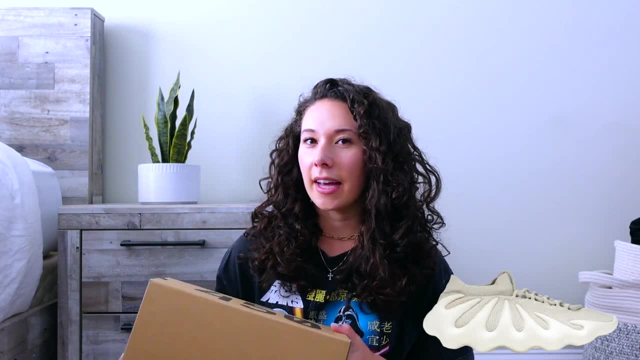 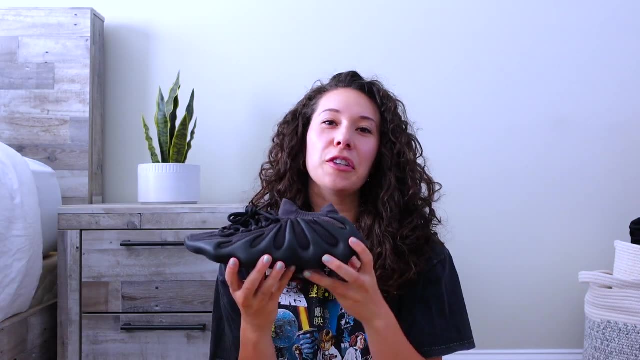 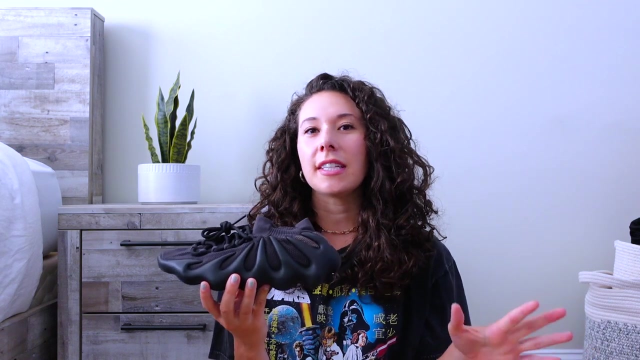 the cloud white and even though it's cloud white, it's kind of like that tan colorway. So these are my favorites. Okay, so here is the shoe and it looks really small, like it's very lightweight, but it does have a little bit of weight, I feel like. just seeing them online it kind of makes me think. 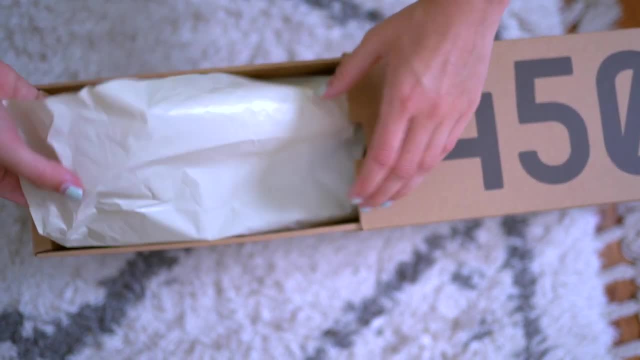 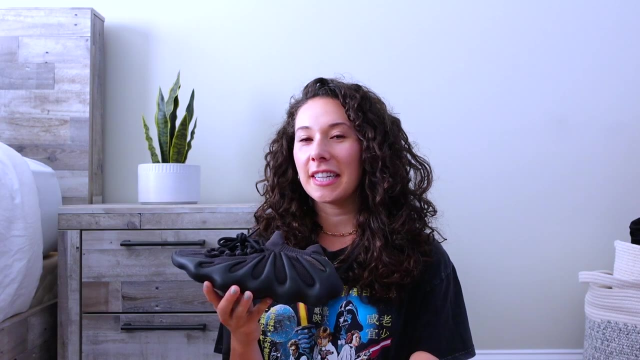 that they would be like extremely lightweight, but the only weight to them is the obvious foam that you can see, So it is still pretty lightweight compared to other Yeezys. and an interesting detail that I noticed is when you first open the box it does smell a little bit different. 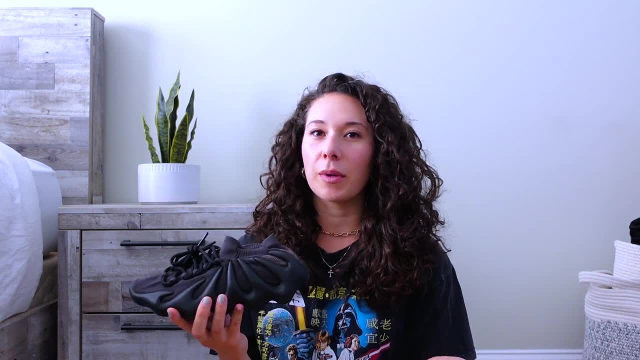 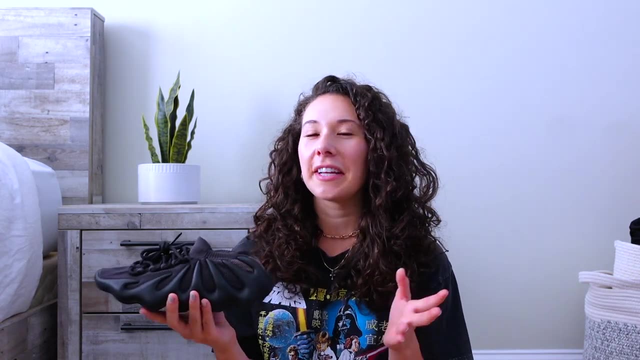 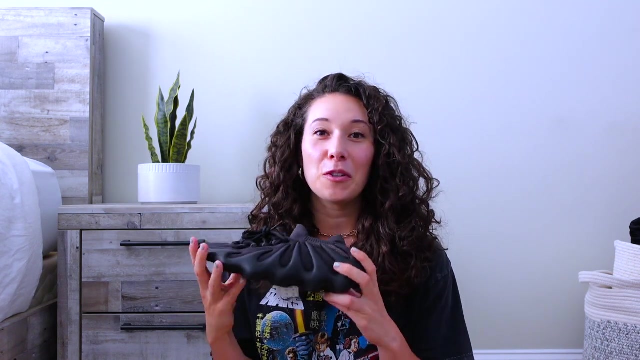 than usual, Yeezys. I mean, I don't really notice a smell with other ones, but this I can kind of smell like it's deeper. It kind of smells like chocolate, like a chocolatey hazelnut thing. I feel like that sounds so weird, but I don't know what it is. It just smells so different. So yeah, let me know what. 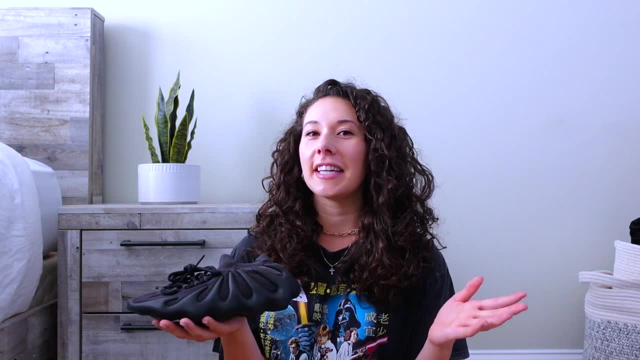 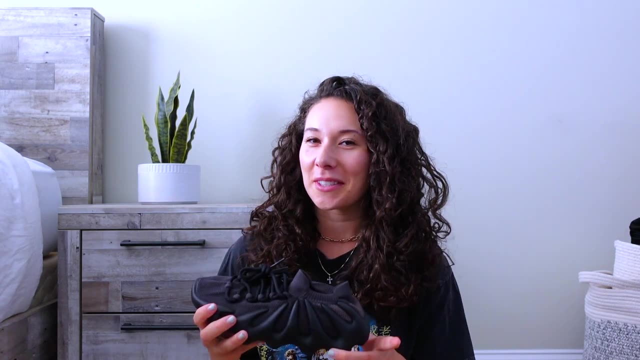 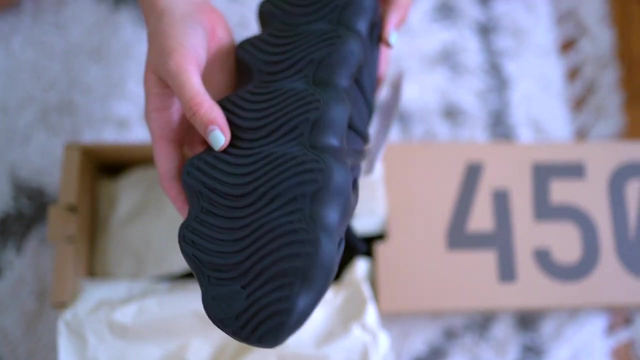 you guys think if you have them, like what they smell like. I can't exactly pinpoint the exact name of like what I'm thinking of, but I just think some chocolatey hazelnut thing sounds good. It's really hard to get used to. It's so different than the typical Yeezy model that we're used to. 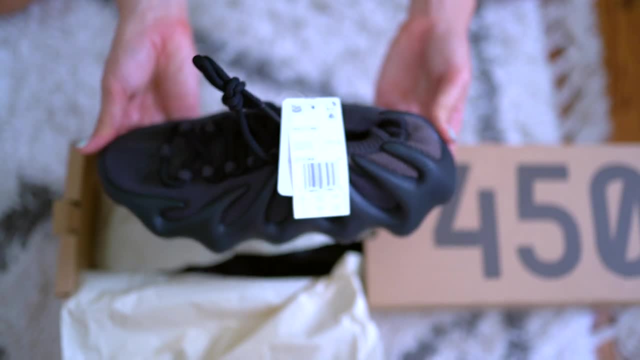 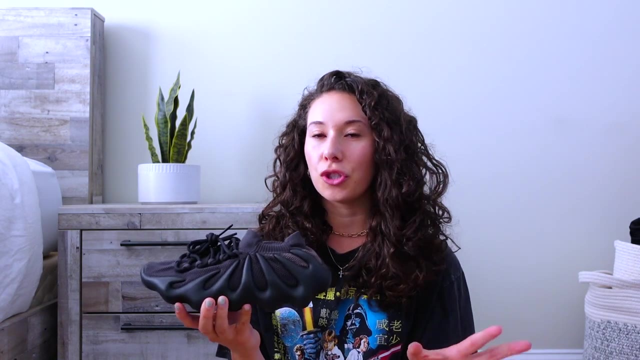 but I do like it because it's really different and if you like a unique shoe, then I feel like it's a good one to have. So basically, the shoe is kind of like compromised, of like two materials and then the laces, and kind of like basing it on the photos online. I did think it would be a little bit. 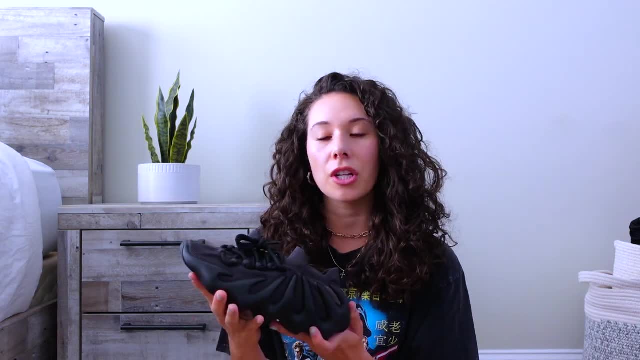 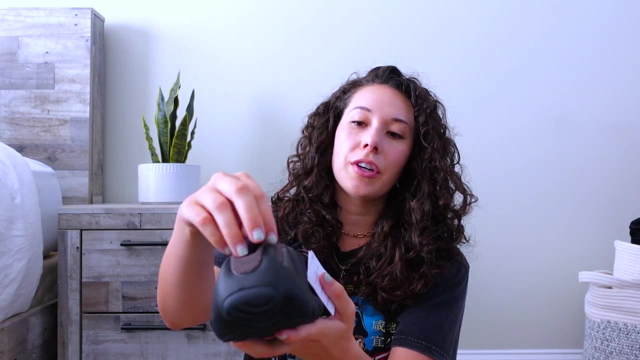 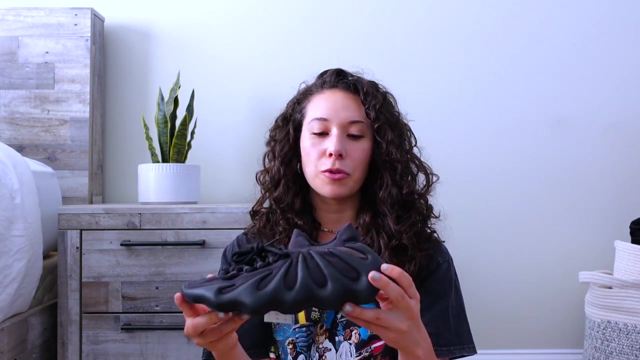 darker in color, but the color does remind me of the cinder colorway. so it's kind of like that brownish black color. I don't know if you guys have seen the cinder colorway, but it's kind of like a tan or a lighter brown color. so there is like a few different browns on here, or just two, and then 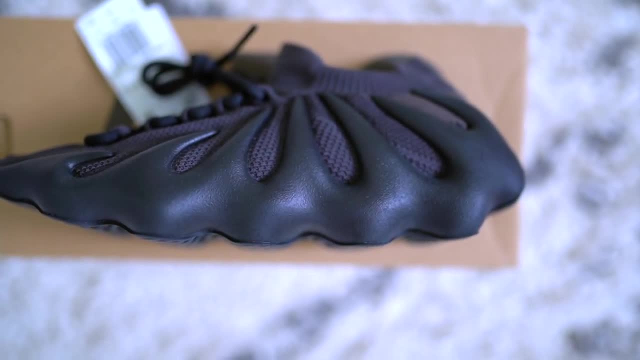 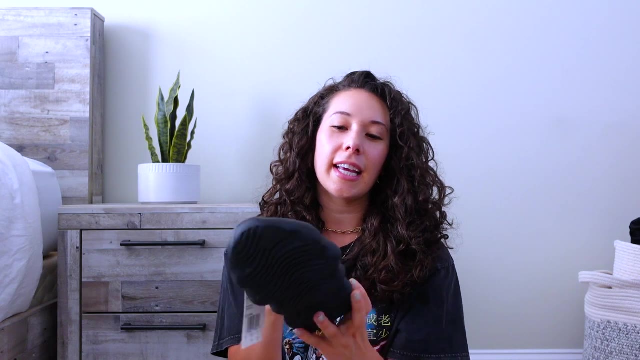 the obvious factor of this shoe. you can see the foam detail is on the sides and goes throughout, and then you also have a sock like ankle grip here. so it's really like easy to put on. It just like slips right on, but it is a little bit tight, and then on the front it does have black laces. 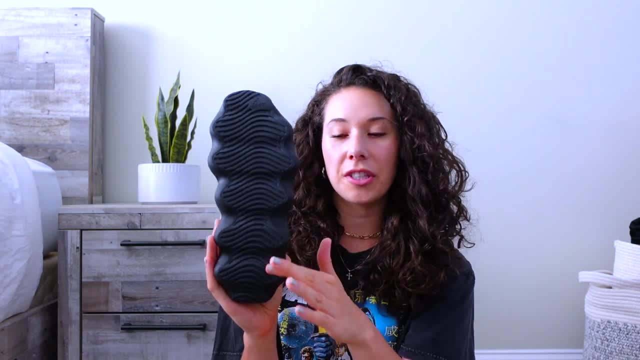 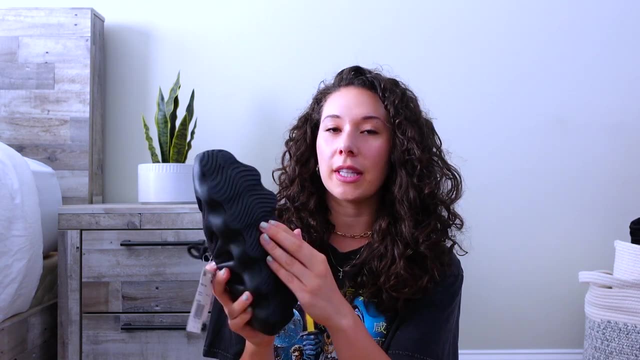 it's like a really nice grip. There is kind of like these wedges in here, so it does give it like a nice comforting feel and it does kind of feel a little like rubberized. so at least you have like some grip right there. and then, if you can see, there's like a little adidas sign like kind of. 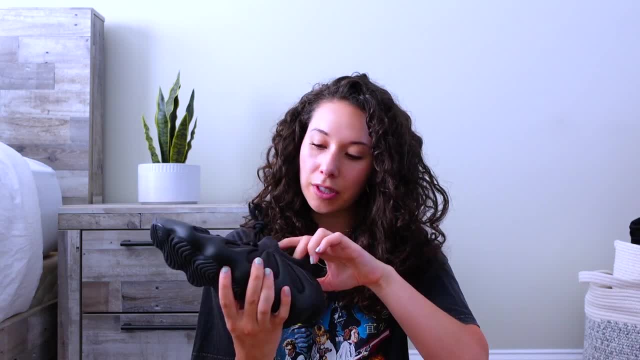 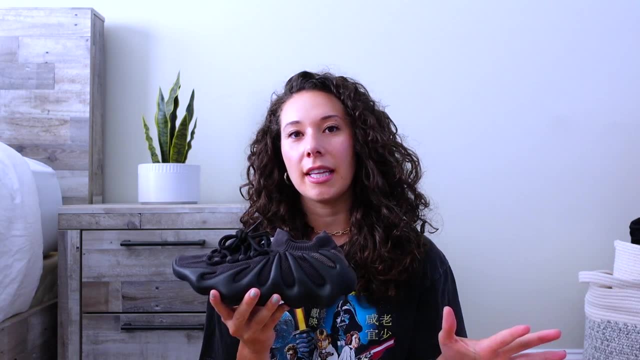 wedged in there and then on the inside of the shoe it does say Yeezy Ortholite. so these are a little bit different too, because they aren't that boost material. so this is more in line with the 500s, and because it doesn't have the boost, I'm assuming it's going to be a little bit more of a boost. that's why it retails for $200, just because usually it is a little bit more for Yeezys with the boost. but the 500s do also retail for $200, so I'm assuming that's probably why. Okay, so for sizing for these they do recommend to go a half size up than like your usual size. 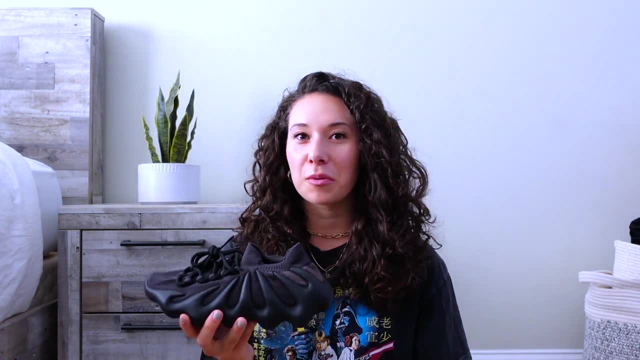 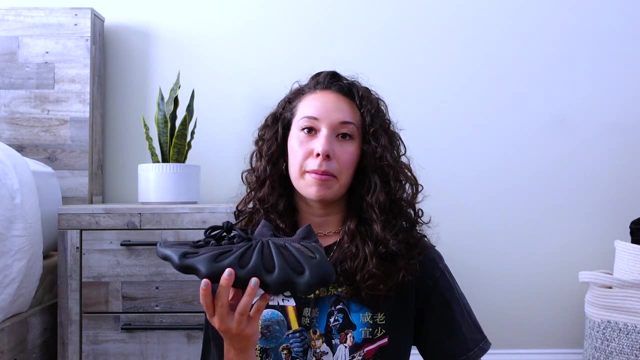 so for me. I'm a woman's eight and my usual size would be a men's six and a half, so I did go ahead and get the men's seven, and I do think that the sizing that they recommend is for the women's eight and the men's six and a half, so I did go ahead and get the men's seven. 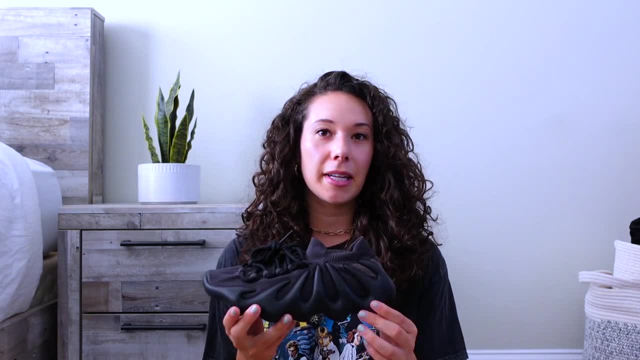 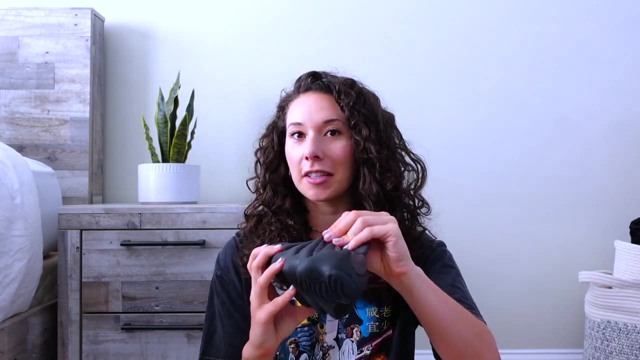 probably the best to like do because these kind of seem like they run small. so I'm happy I went with a size seven. like getting the shoe on it's a little bit tight because obviously it's like a sock like material, so it is a little bit tight like putting it on, but once it's on it does fit. 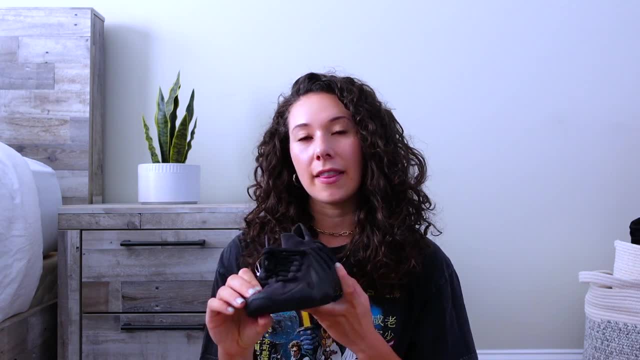 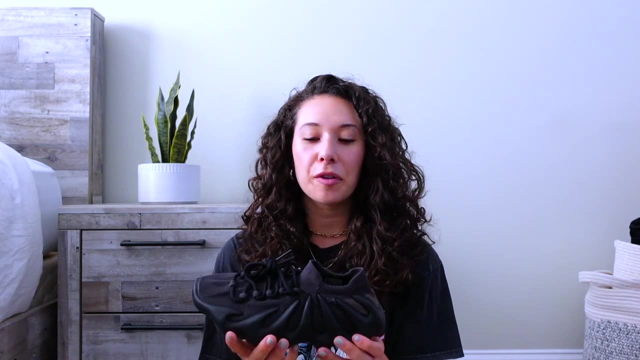 really nicely. I do have a little bit more room, like in the toe box area, but it's like just enough, so it's perfect. so, yeah, I do think that the half size up is perfect, but I mean, you probably can get away with going truly half size up, but I do think that the half size up is perfect, but I mean. 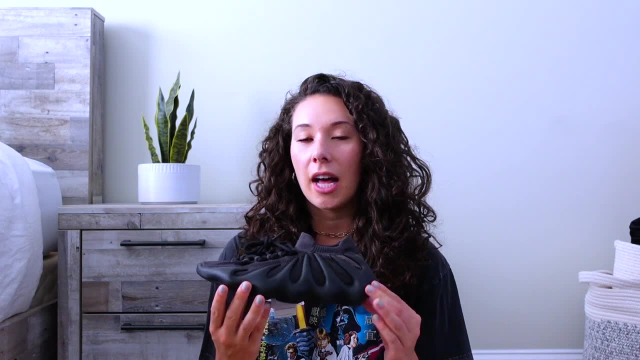 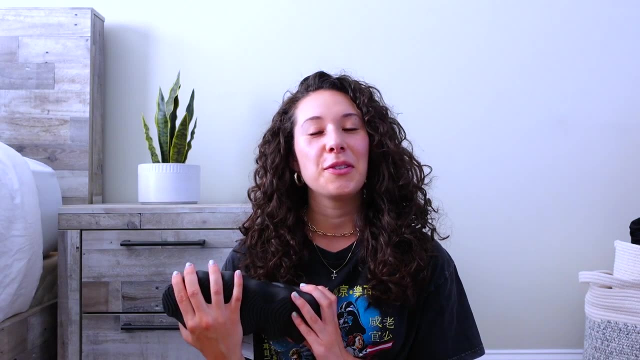 if that's what, like you usually do with Yeezys, but I would just base it off of, like what works best for you, but for me the half size up was perfect, okay. so before I get into the on feet, I do want to just like give my opinions on this shoe and like what I'm thinking about it. 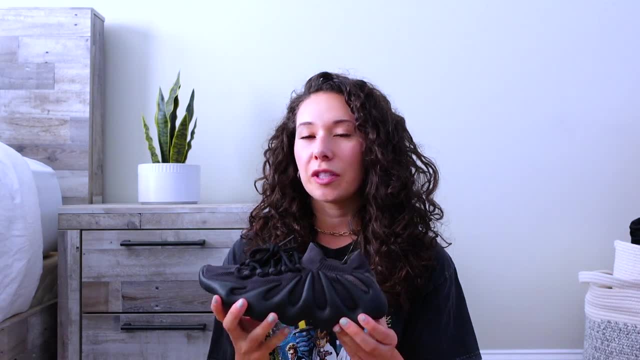 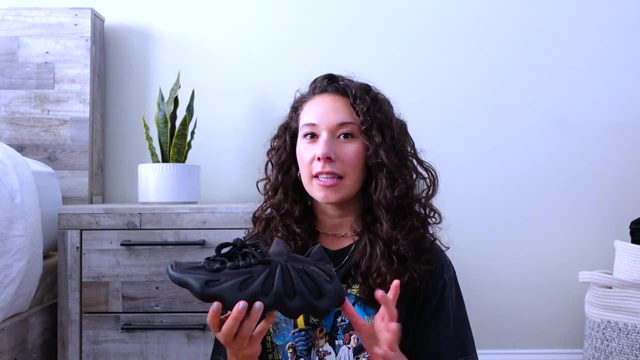 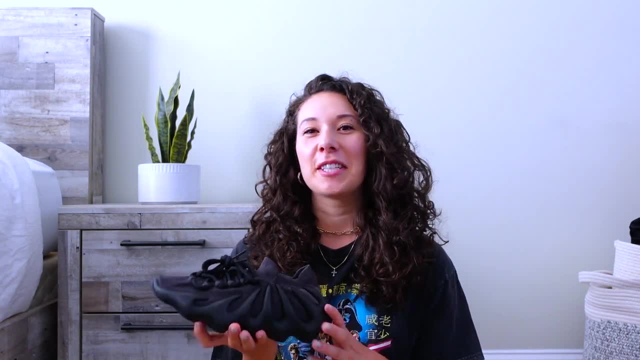 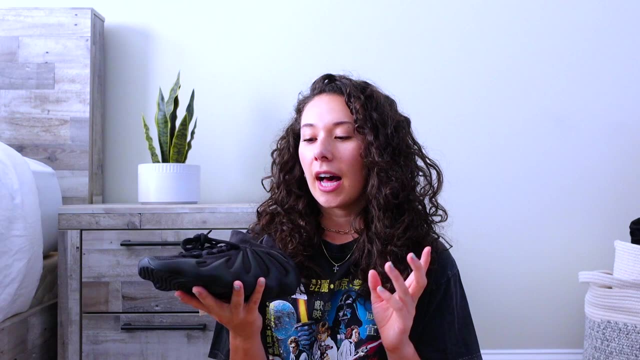 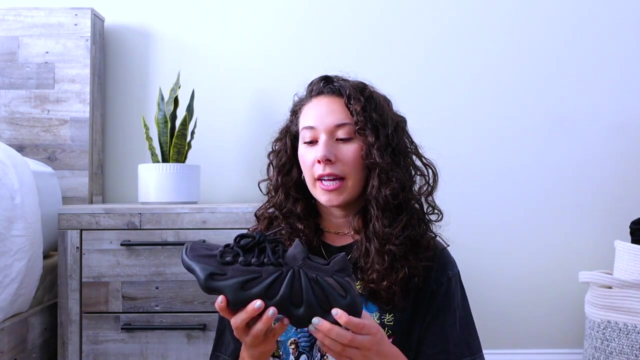 like I really like that. a lot like comfort is everything, especially with Yeezys. the only thing is it does kind of look a little bit weird, so I feel like it is hard to style. I do think that maybe the cloud white would be a little bit easier to style, just for me personally. but if you're like 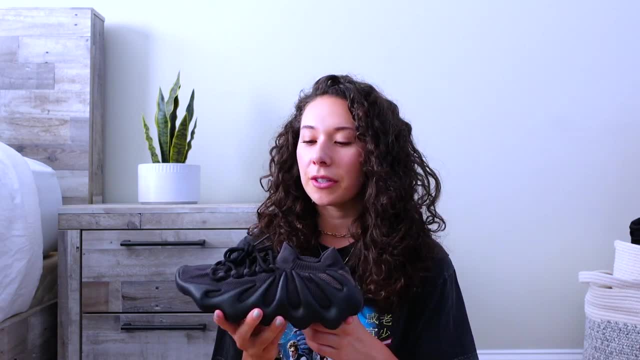 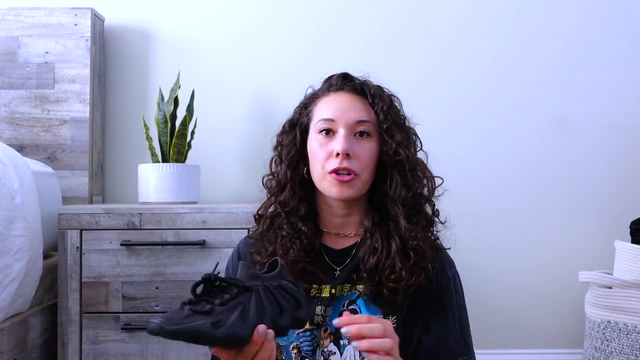 looking for an all black shoe, then this colorway would be a little bit better. but also just keep in mind it does have the like hints of the brown, just because in the photos it kind of looks a little bit darker than maybe it is in person, but I do think that it's a little bit better.